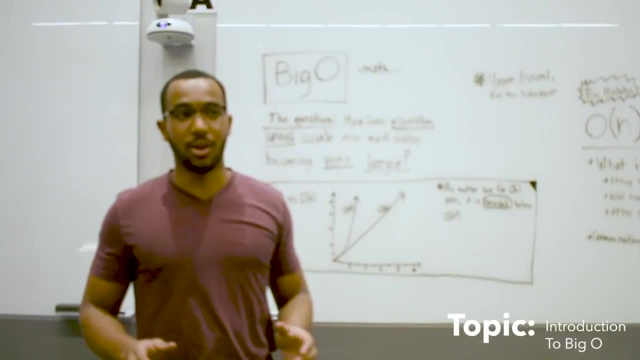 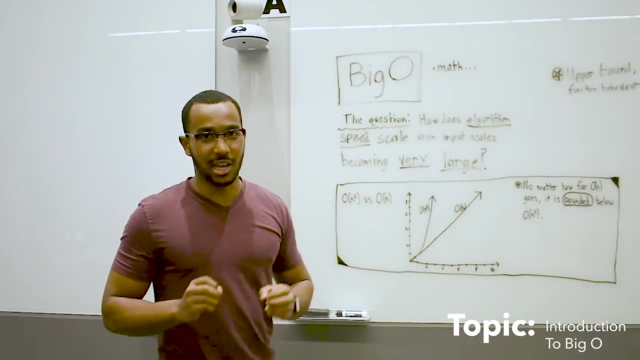 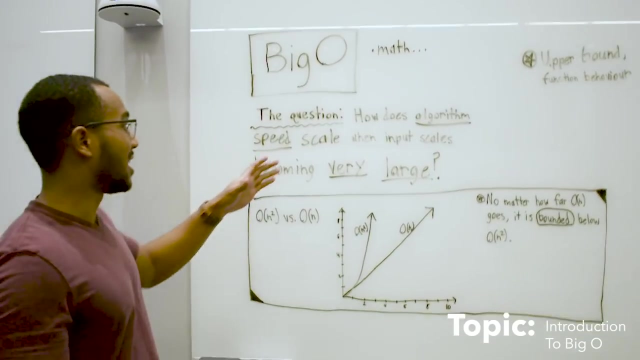 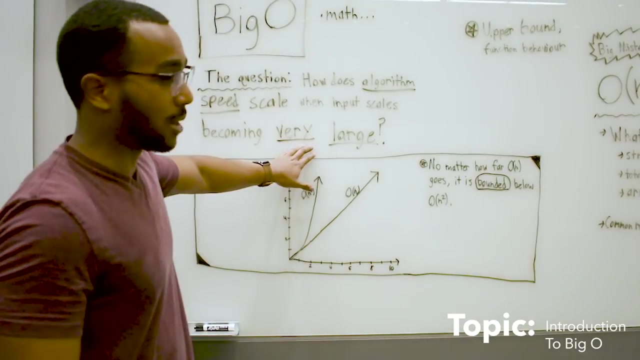 And so there's a mathematical definition for Big O Notation and it talks about upper bounds and sometimes it confuses people, but there's a root concept that you need to understand when you think about calculating algorithmic time complexity. So we ask ourselves a really key question. We ask ourselves: how does an algorithm's speed scale when input becomes very large? And very large is the key term here, because, for an example, here we have a function that runs in n squared. 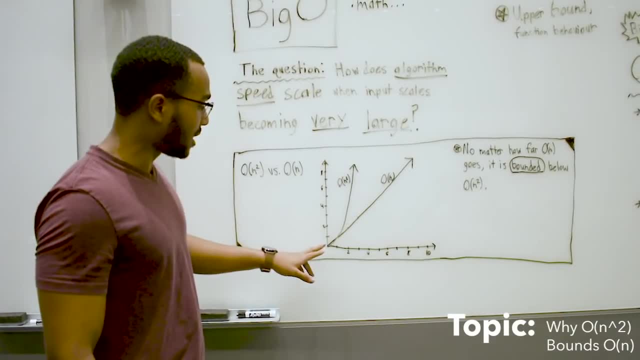 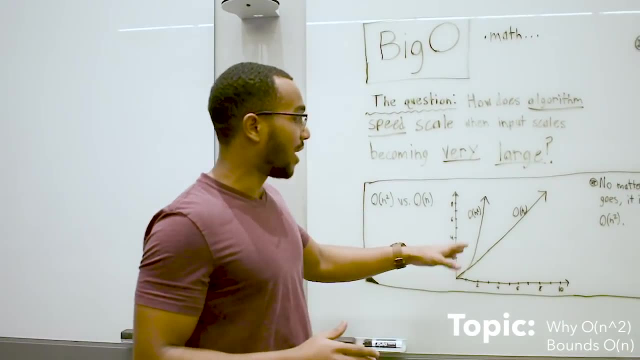 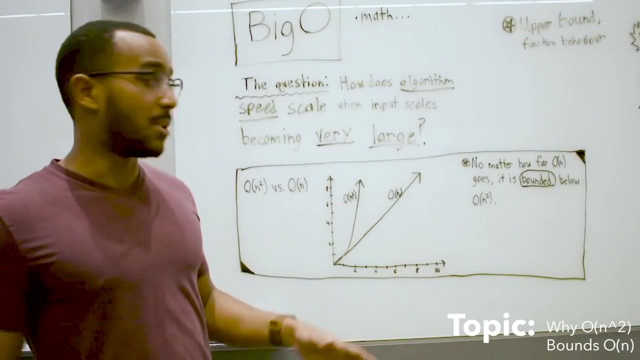 and a function that runs in linear time: O of n. So, as we can see, the O of n is actually actually O of n squared is faster at the start versus O of n, but what you see is, as input becomes very large, the O of n? squared algorithm has a much longer run time than the linear time. 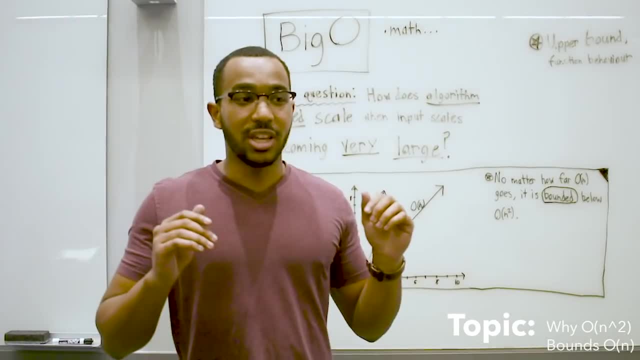 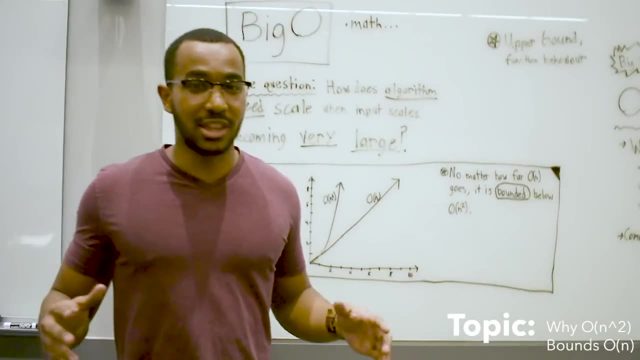 So this is why it's called asymptotic complexity. It's looking at tail behavior, It's looking at the literal behavior of a graph as input scales very large, And that's a very important thing, And that's a very important question when you're thinking about algorithms and optimization. 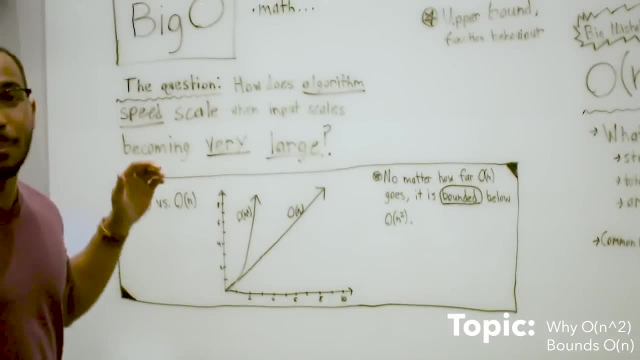 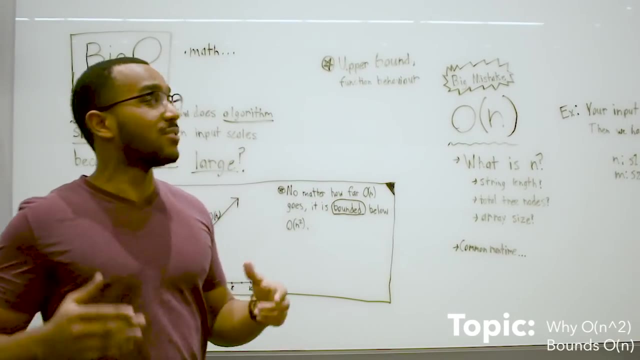 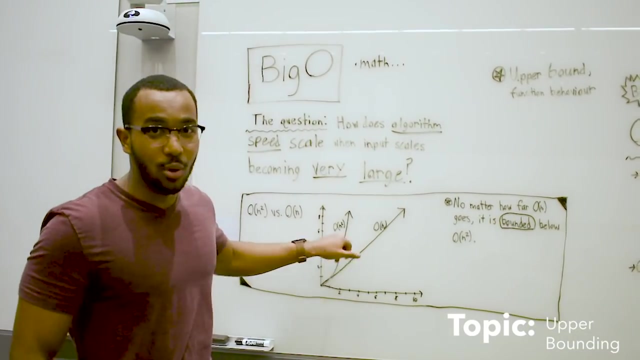 So, no matter how far O of n goes, it's going to be bounded by O of n- squared, and bounded is a very key term. So what O of n, what Big O, gives us is a very tight upper bound to functions. We know that this linear function is not going to go past an n squared function as input becomes very large. 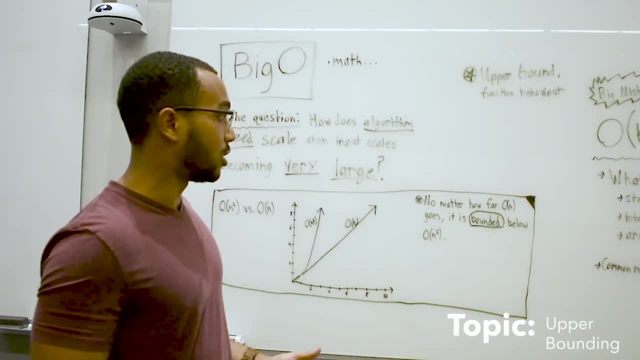 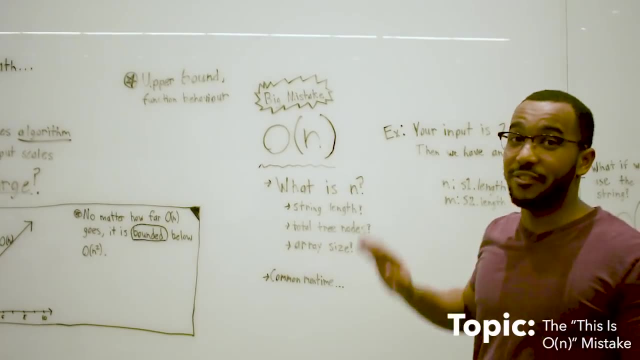 We know that the linear time function is going to be faster as input's very large. So here's a very big mistake that's made with run times. O of n. linear time is a very common run time, But what is n? Is n the string length? 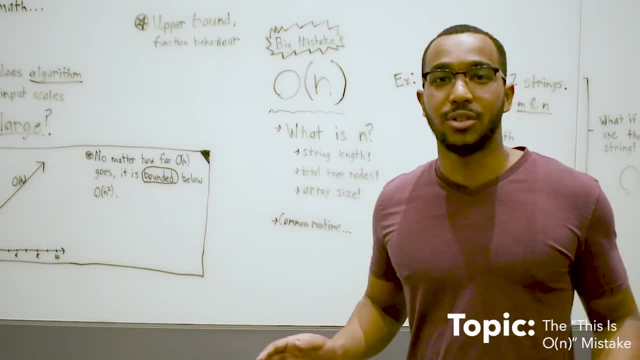 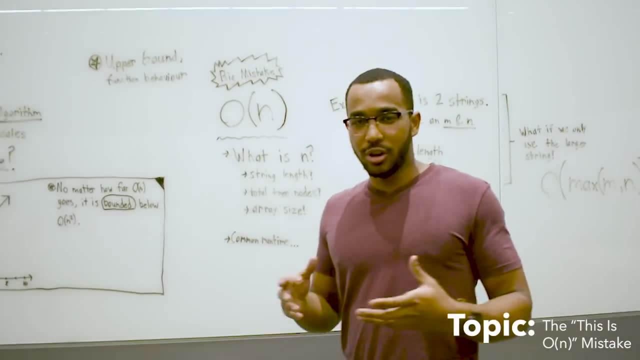 Is it the amount of tree nodes? Is it the size of the array? What is n? And a really key thing that an interviewee needs to do is define what is n. What are your variables? What are you scaling? What is your input? 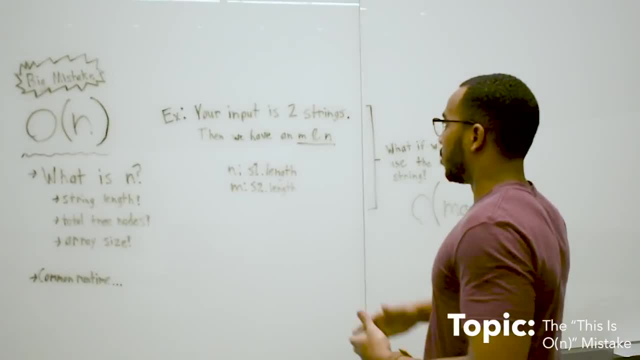 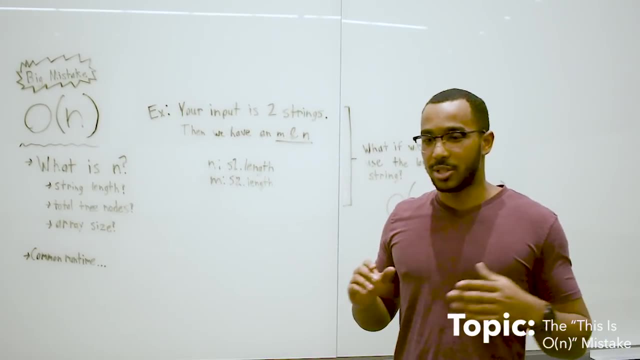 This is very important. So let's take an example. If you have two strings Instead of two strings of input, our run time is not O of n. This is a very common mistake. It would be O of m, and then you have to factor in n. 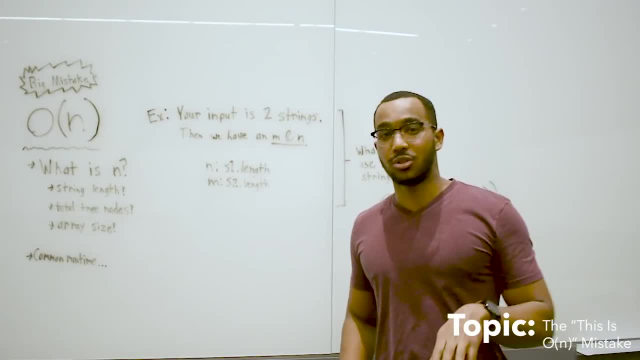 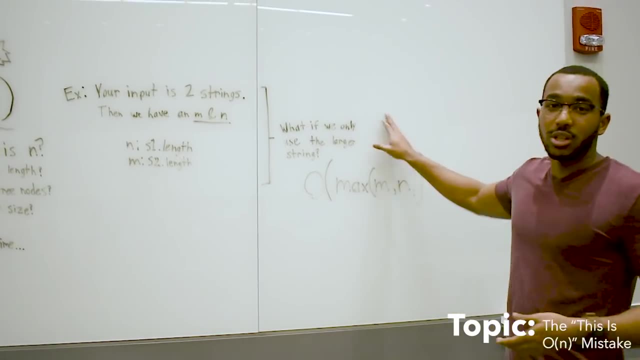 So n would be the first string's length and m would be the second string's length, And it might be m plus n. it might be m times n, It depends what the problem is. So what if we're only using the larger string? 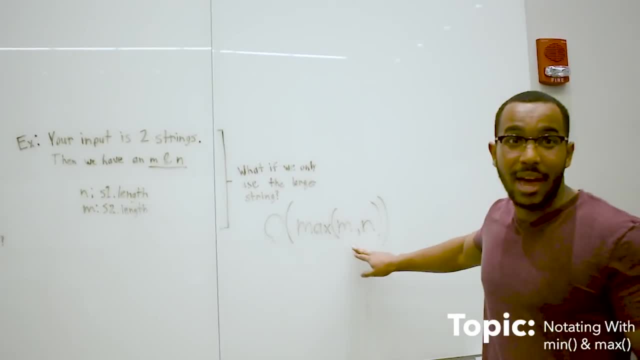 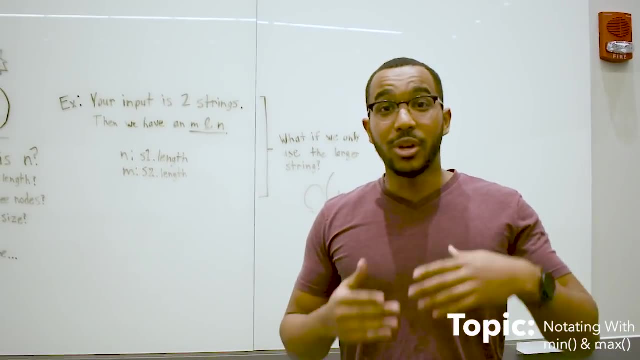 Then we get into min and max notation where we say O of max, m and n. So if we're just taking the larger string, we don't know whether we're taking m, we don't know whether we're taking n, but we know we're taking the larger one. 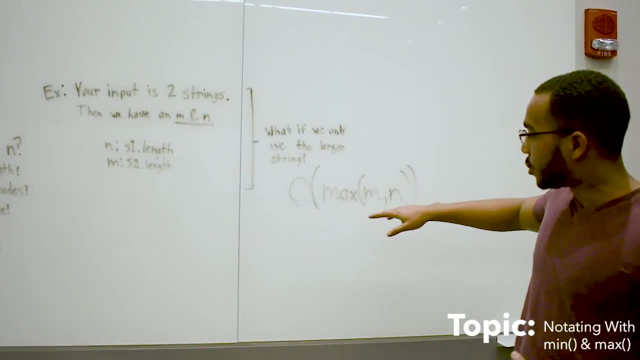 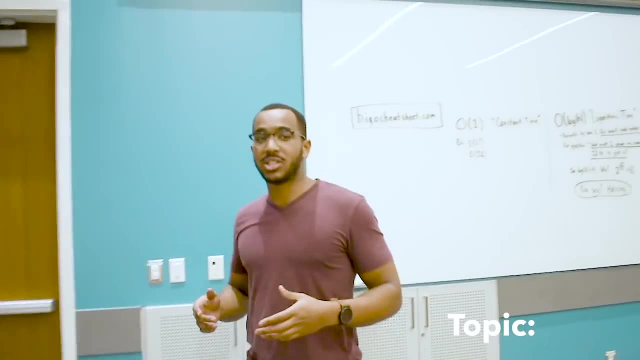 We know we're taking the max of them, So we can use this notation here to say this is what we're basically doing. That's a shorthand, So, moving on, we're going to look at the common time complexities that you'll see in different kinds of problems. 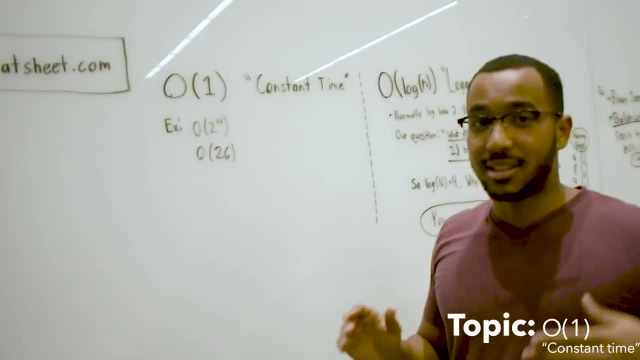 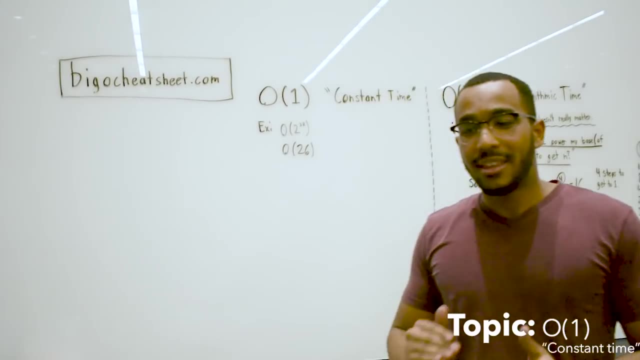 So the first time complexity is constant time. So what does constant mean? Constant time means that as an algorithm gets very, very large input, the runtime of the algorithm stays the same. It could be O of 26,. it could be O of 2 to the 32,. 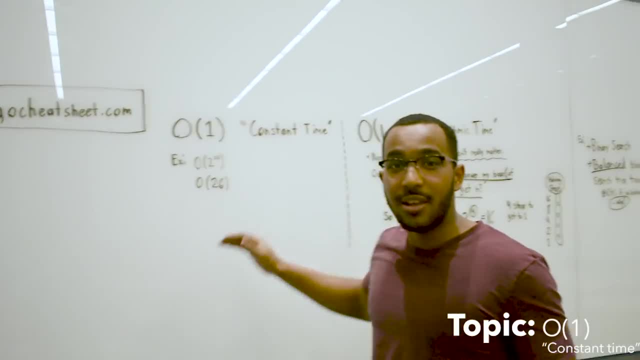 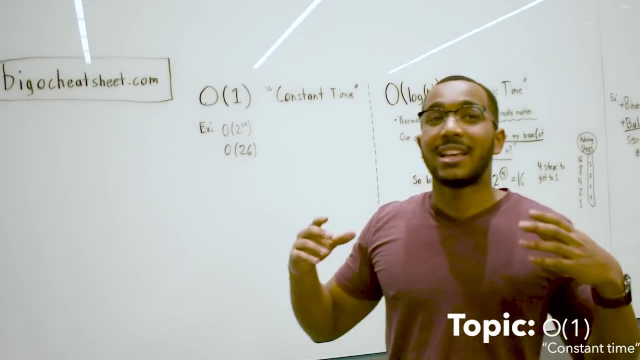 as long as it's constant, As long as it's a constant line, that means it's constant time. It doesn't matter how large that constant is. What we're worried about when we think of big O, we're worried about tail behavior, the form of a graph. 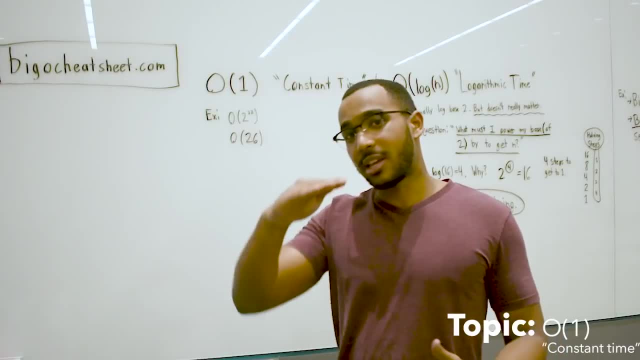 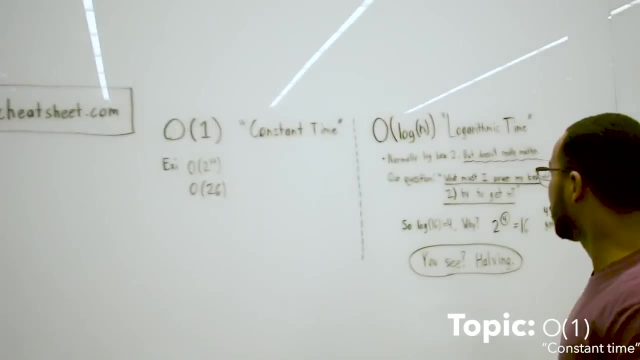 the way something scales And what constant time looks like is, as input gets bigger, that line stays level. The runtime of the algorithm does not change, So then we get to log n time. This is something that really confused me a lot, because I wasn't good at logarithms when I took calculus. 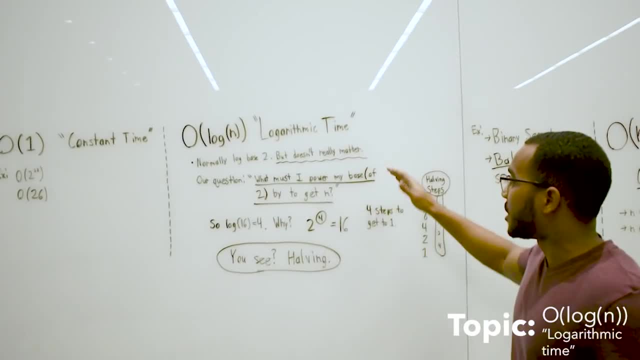 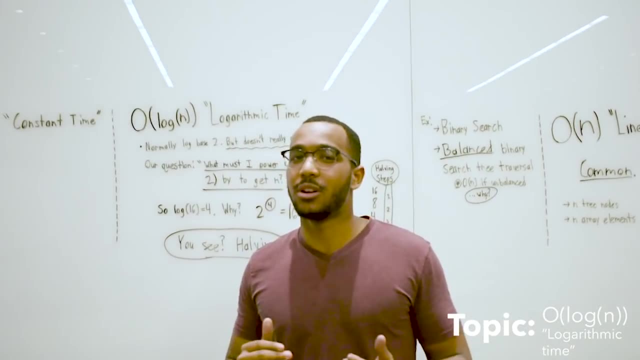 And we call this logarithmic time. So normally it's base 2, but we care about the behavior. Again, this is the number one thing I have to stress. Logarithmic behavior looks like a logarithm and it grows kind of like this: 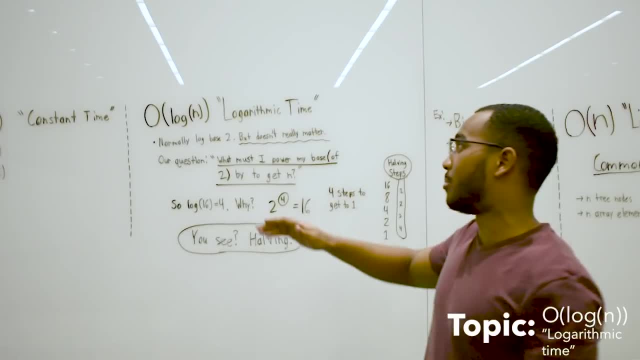 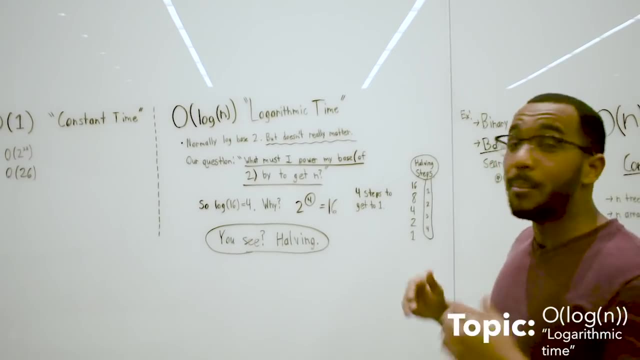 So the question that a logarithm asks us, fundamentally, log base 2 asks us, is: what power do I need? What do I need to power my base- in this case it's 2, by to get n. What do I need to power 2 by to get the original n. 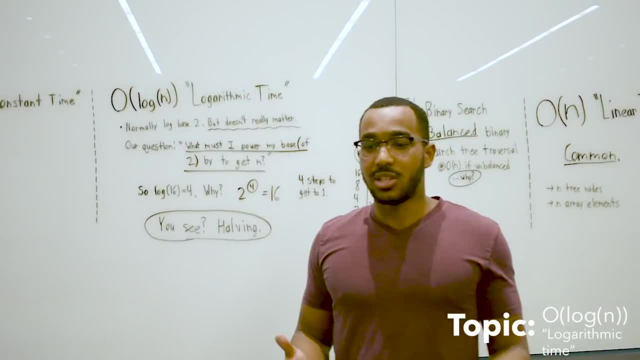 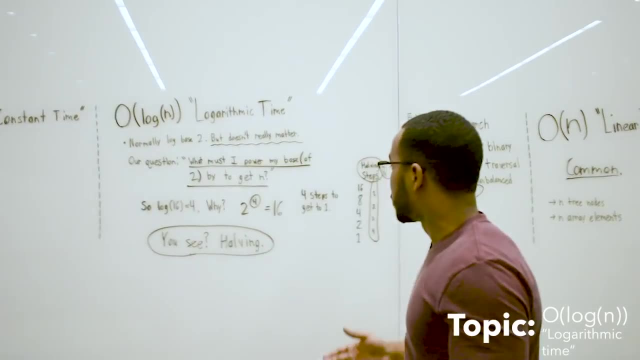 So take for example log 16.. How do we get 16 from 2?? What do we need to power 2 by to get 16?? We need to do 2 to the fourth. 2 to the fourth is 16.. 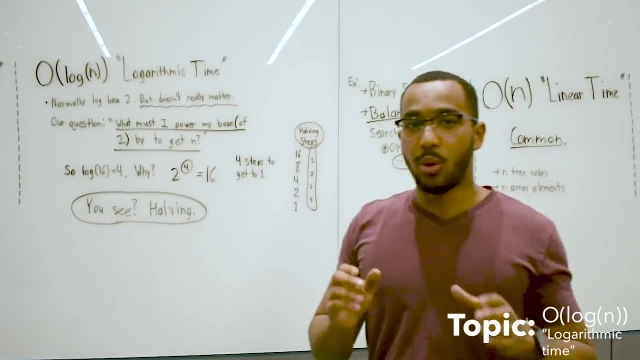 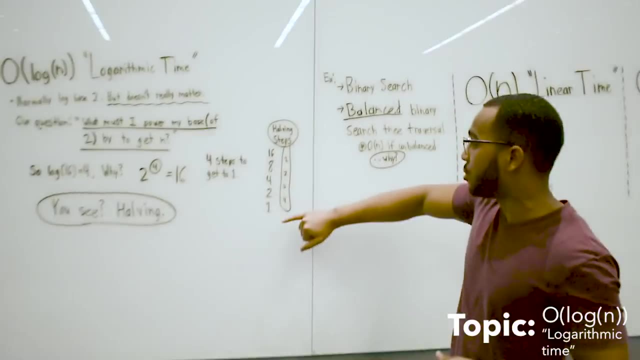 So what does that mean? That means it takes us four steps of having 16 to get to 1.. And, as you can see here, we take 16, get 8, 4, 2, 1.. We see that we're having. 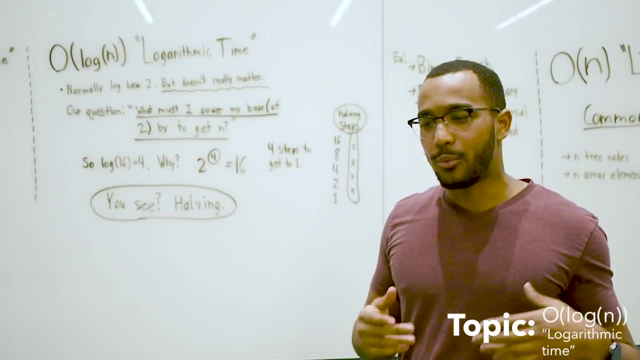 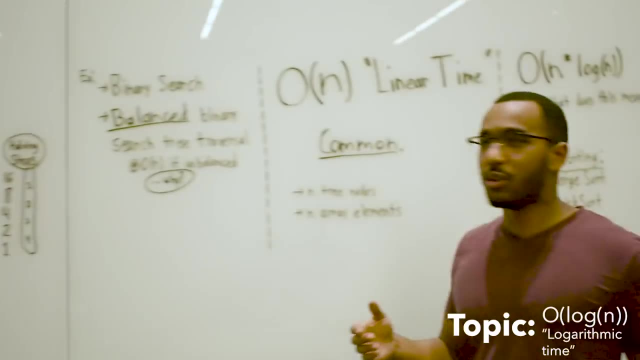 So this is a really key thing me saying having: Where does that factor into? So this is a very key thing. So where that factors into in your algorithms are your binary search. What binary search does? it has the invariant that something is sorted. 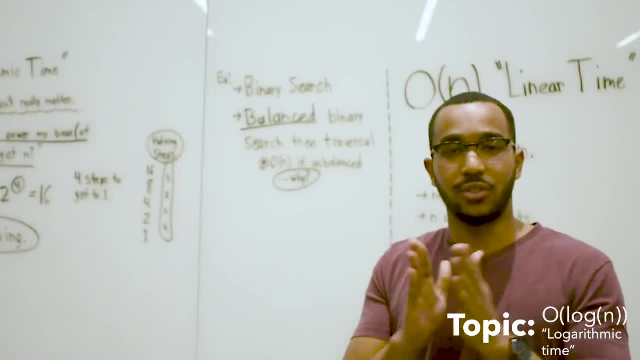 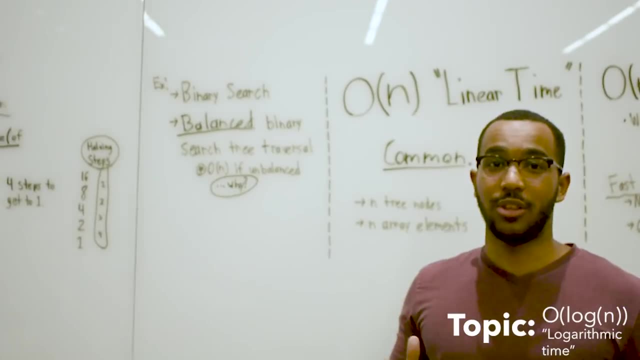 Invariant just means something that's always true within our certain space of searching or performing work. It's the invariant that we can have the search space and keep it sorted. So this is where logarithmic logarithms come into play. We're having our search space. 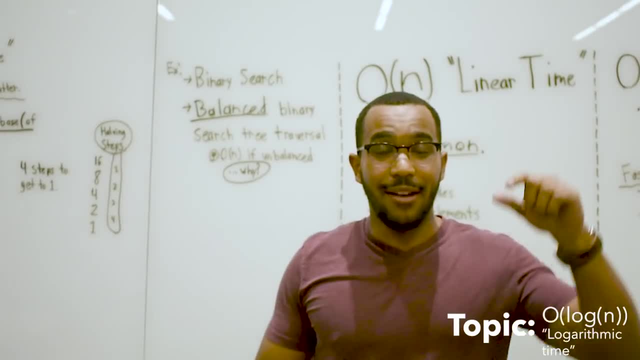 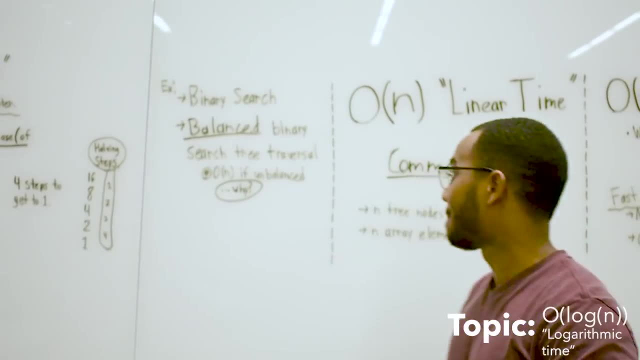 And if we have a binary tree or a binary search tree that's balanced, every time we go down a level we're cutting off a whole half subtree. We're literally having our search space every single time, And this is only if the tree is balanced. 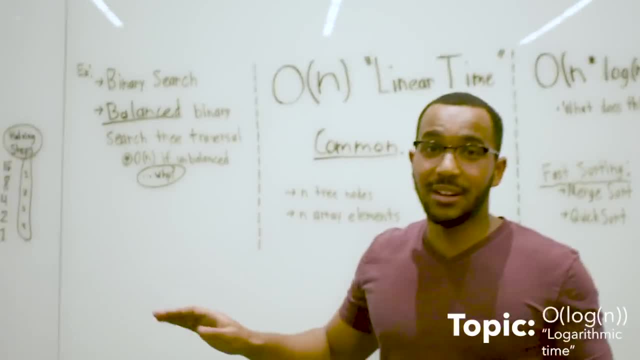 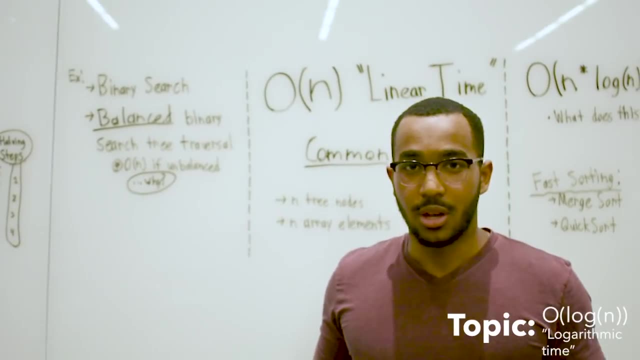 I'll get into doing tree videos later, But it's O of N. if the tree is unbalanced, If it's skewed to the right or left, then it's going to. you're going to be touching all of the nodes, But that's just another detail for another day. 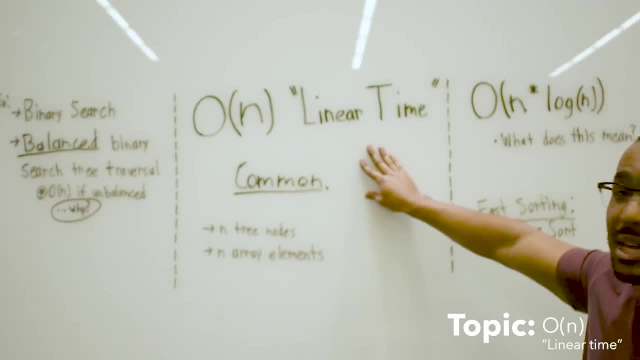 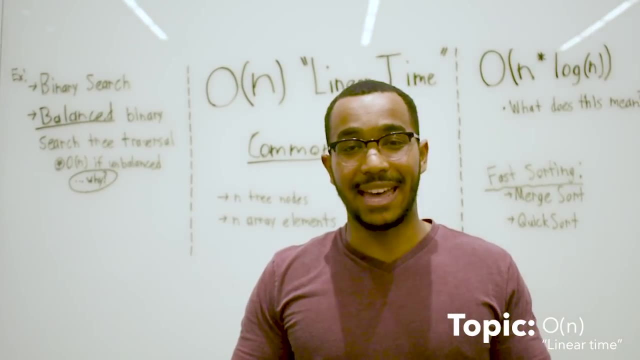 And then O of N time is the most common O of N time is linear time. So, whether you have N tree nodes, whether you have a string length N, an array length N, this is when you're going to see a linear time algorithm. 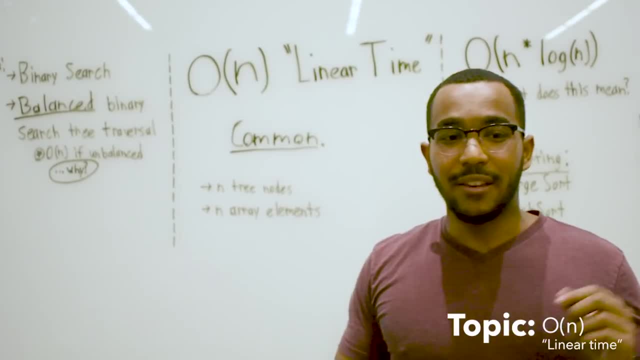 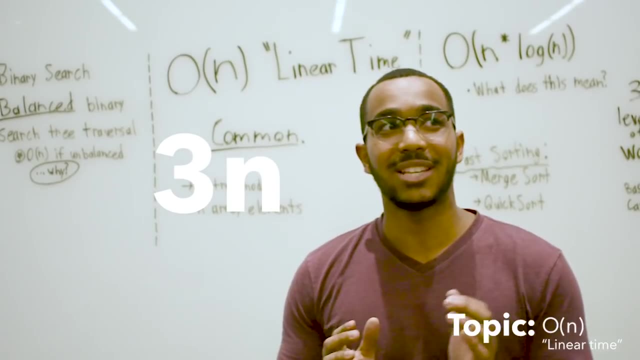 because you're going to be touching all N of the nodes And even if you're doing multiple passes over an array, you're going to be doing 2N, 3N. But what we care about is not the. we don't care about the constants. 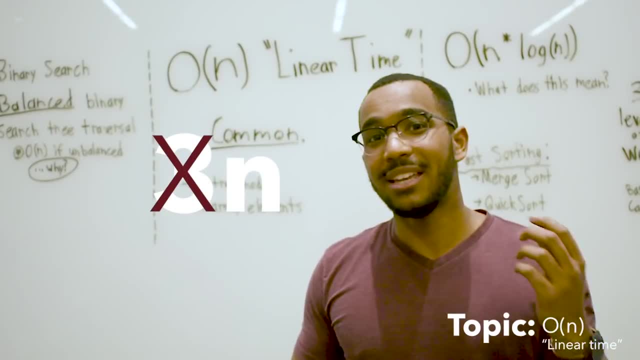 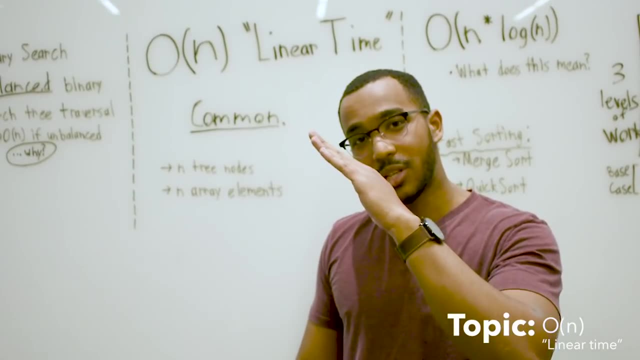 This is why we drop the constants in Big O notation 3, Big O 3N is the same thing as Big O N, because we care about the behavior. The only thing a constant is going to do is going to make that line steeper. 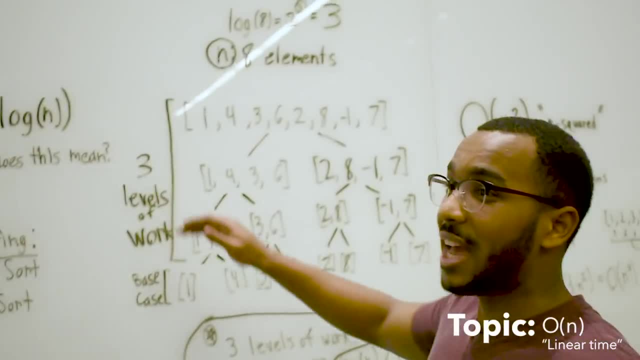 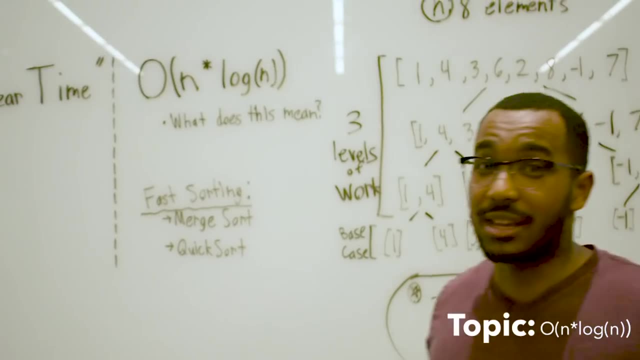 That's all we care about. We care about the behavior, And then we get into. this is one of the more confusing complexities as well. This confused me a lot. N log N. So what is this saying? It could be saying a lot of things. 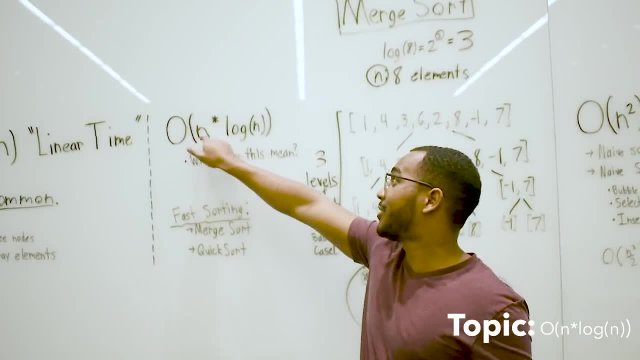 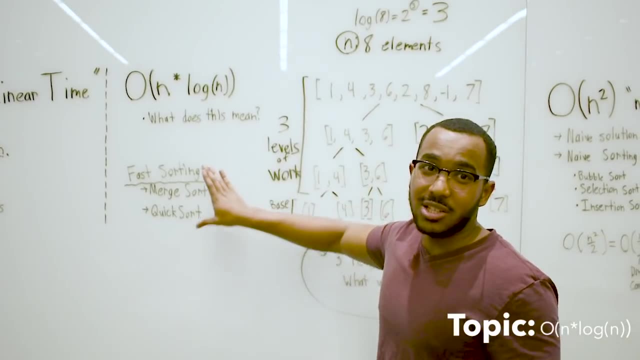 It could be saying we're doing log N work for each of the N elements we have. This is what multiplication does. I'll talk about multiplication addition in another video. So what does it mean? So often we see this time complexity with quick sort and merge sort. 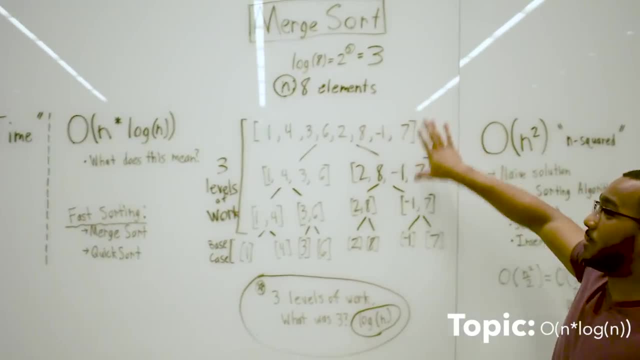 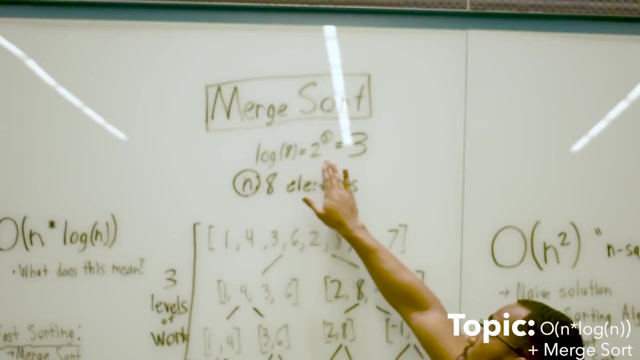 our faster sorting algorithms. So here's an example to run through everything. So say N is 8.. Say we have 8 elements And log 8 with base: 2 is 3.. 2 to the 3 is 8, right. 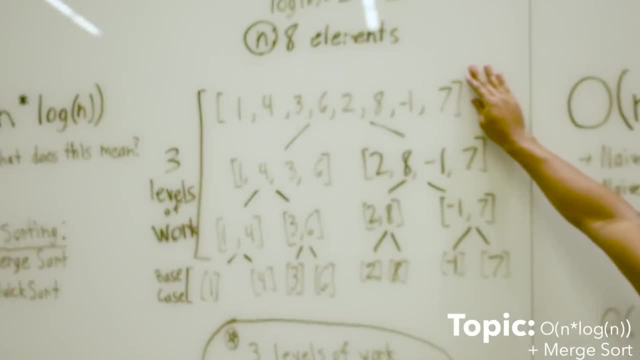 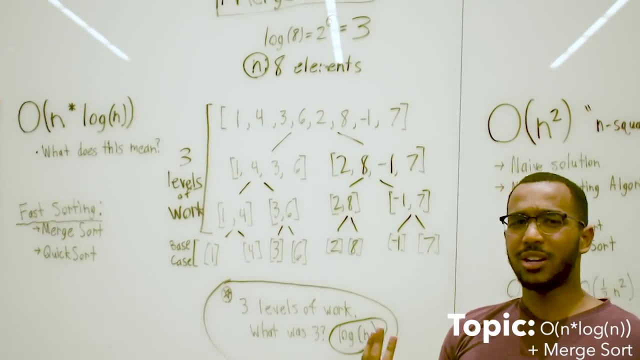 So this is basically how merge sort works. It's going to take our unsorted input, It's going to have it each time, And what we notice here is we have 3 levels of work. And where is this 3? looks familiar. 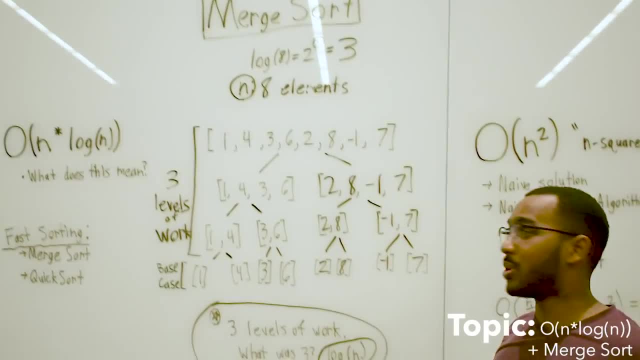 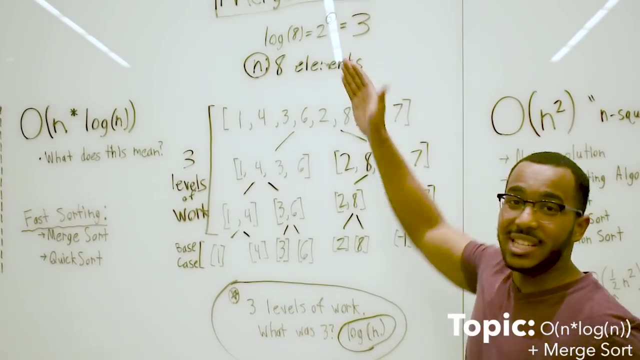 We, literally we just got this 3 up here. That is not a coincidence. So we have 3 levels of work. And why is it 3?? It's because we take the log of the 8, because we're doing halving steps. 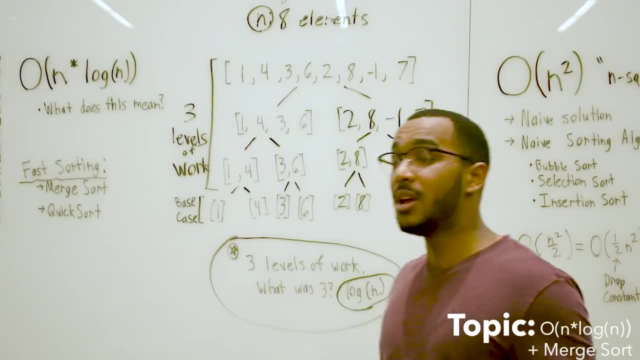 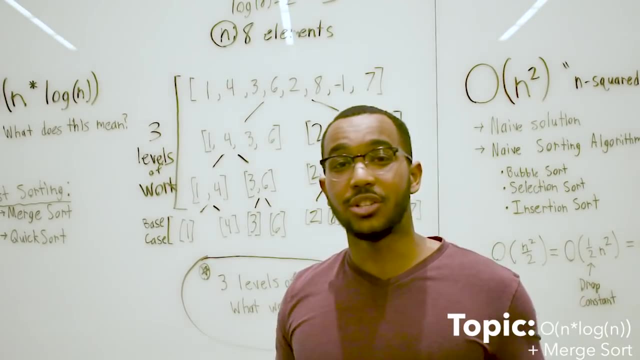 Just like I was saying before, the idea that we're cutting things in half is important. This is where it plays in. So we are cutting things in half And we're going to have log N levels And for each of those log N levels, 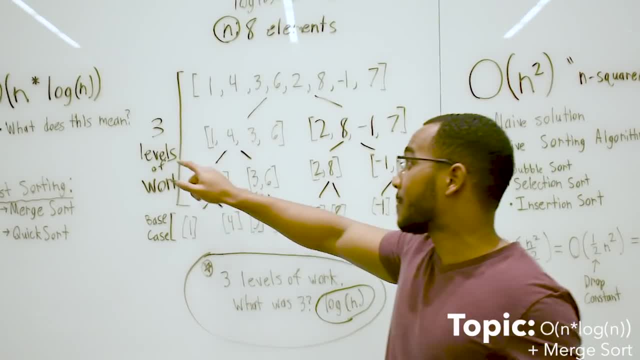 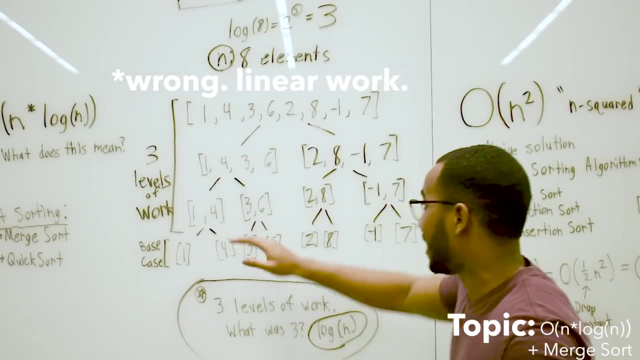 which in this case are 3 levels, because log 8 is 3, for each of those 3 levels, we're going to be doing constant work. We're going to be touching all N elements in each level to be merging these on the way up. 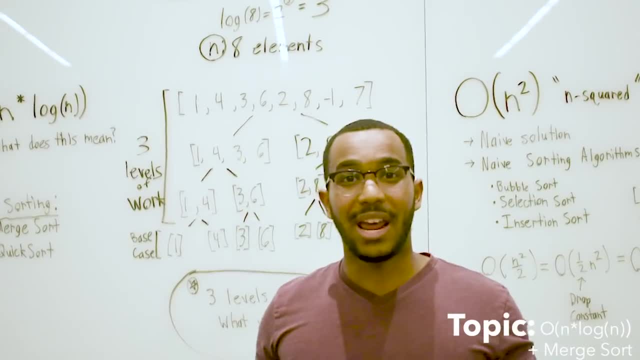 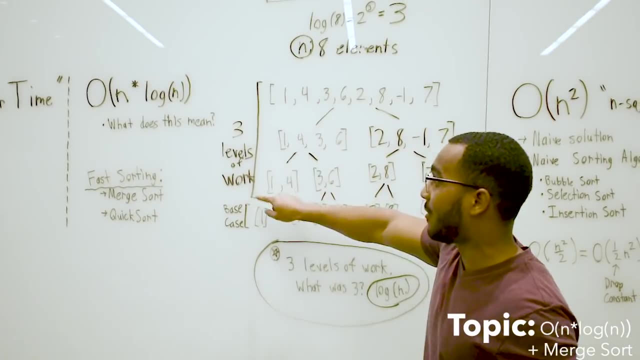 I'll get into specifics of merge, sort and quick sort in another video and how the recursion builds back up, But this is very fundamental. This is a good way to understand this complexity, because we have log N levels and we're doing constant work in each level. 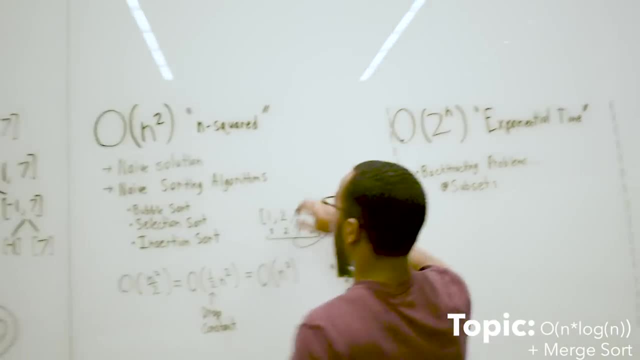 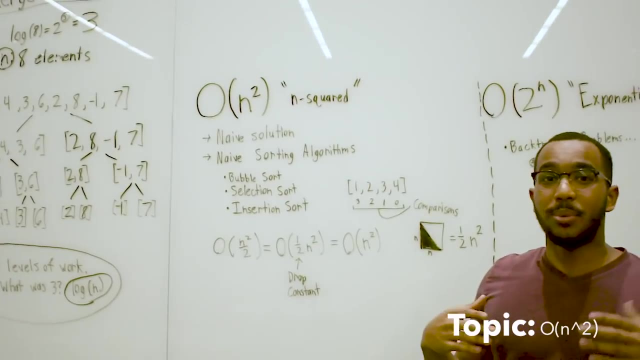 So this is kind of like what you should be visualizing. So next we have N squared. Any time you see N squared, it's always going to be probably the first naive solution to a problem And it's going to be our more naive sorting algorithms. 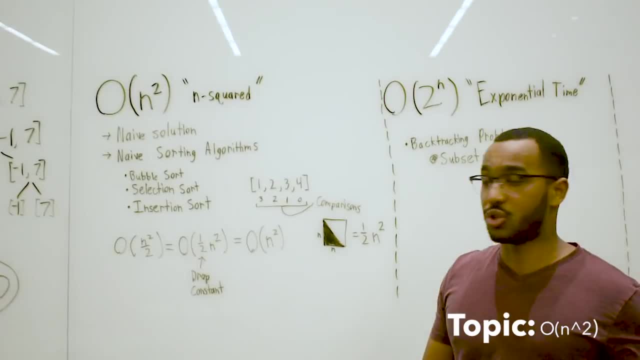 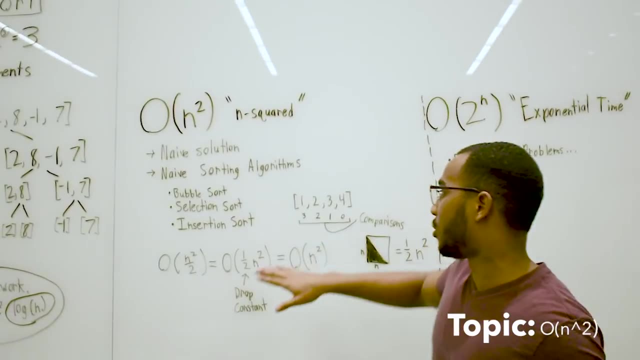 Things like bubble sort, selection, sort, insertion, sort. So one thing that you'll notice is, even if you have a normal array, so something like this, with 1,, 2,, 3,, 4,, if we do 3 comparisons for this index, 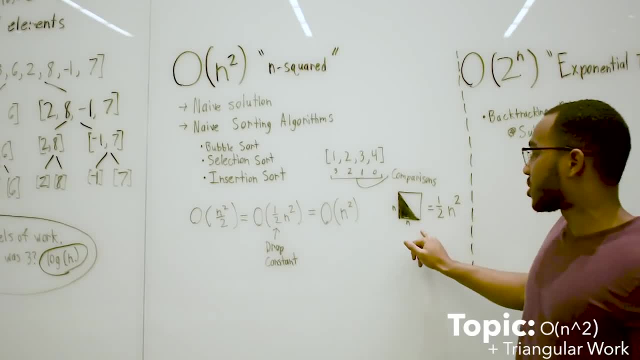 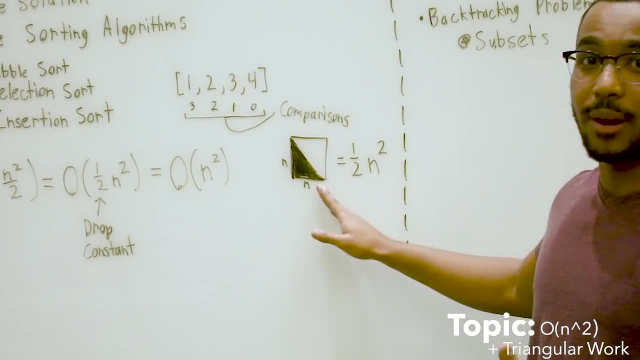 2 comparisons: 1 comparison, 0 comparison. it forms what looks like a triangle, And what this triangle is cut out of is a square. So what is the square from? We have N by N, That's N squared, And we're taking 1 half of it. 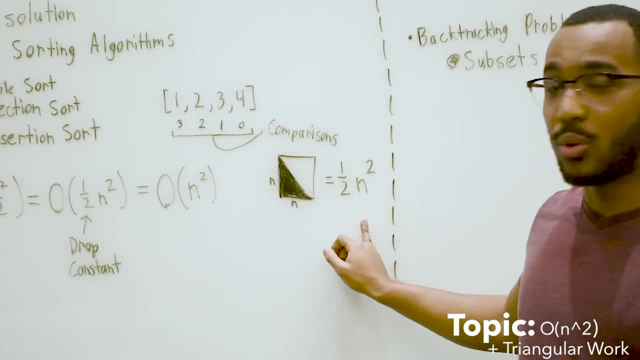 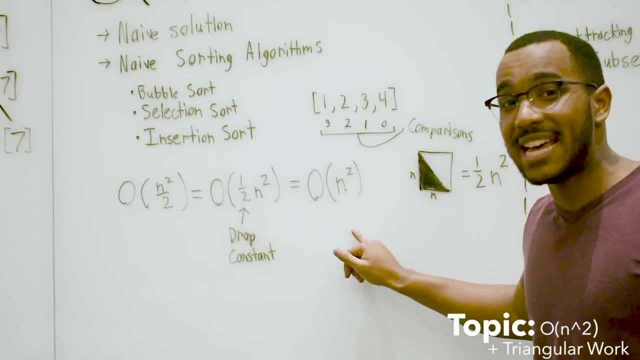 So, even if we're doing something like this and we're taking 1 half N squared, what do we notice? We notice there's a constant right there. And what do we do with constants? We drop constants because the behavior stays N squared. 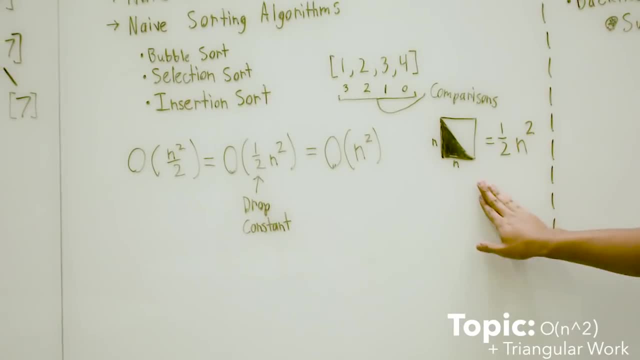 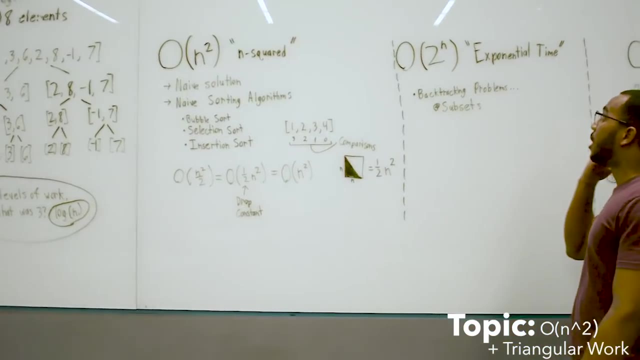 So things like triangular numbers and things like that, those end up being N squared anyway, although they end up making a triangle of sorts with their sums. So that's another thing to look out for. And then we have N squared, We have 2 to the N. 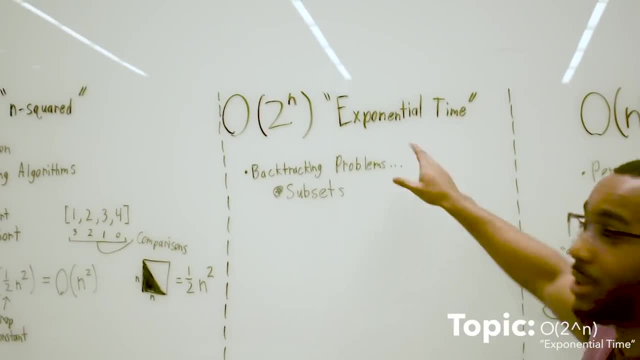 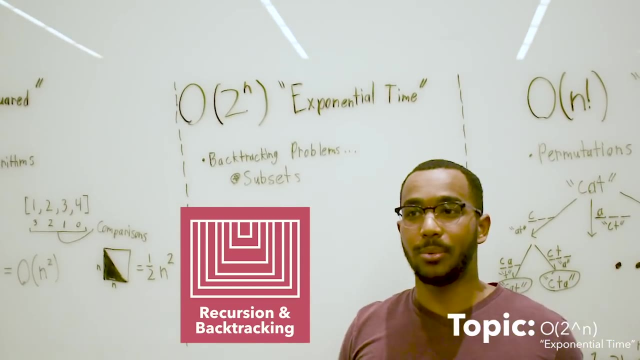 It could be 4 to the N, It could be 6 to the N. We have exponential time. So exponential time, we normally see that when we have backtracking problems, recursive problems that are creating forks And for each of those forks, 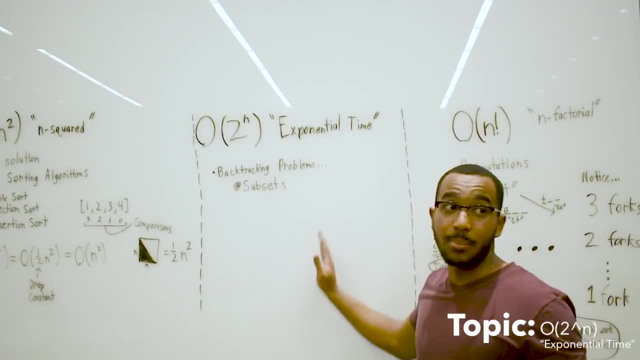 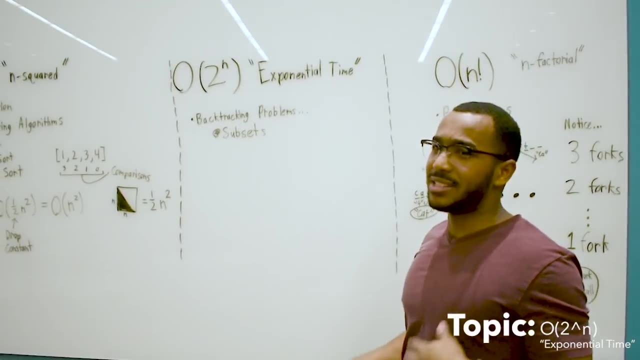 we're creating two forks and we're going to have N levels deep. We'll look at that when we look at the Fibonacci over there. But problems like this are like subsets and different backtracking, recursive problems we'll get into. And then finally, we have factorial time. 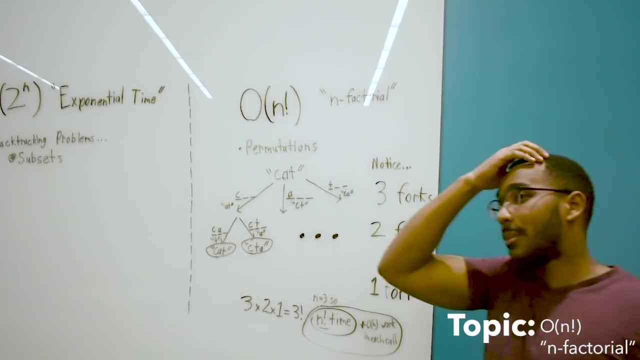 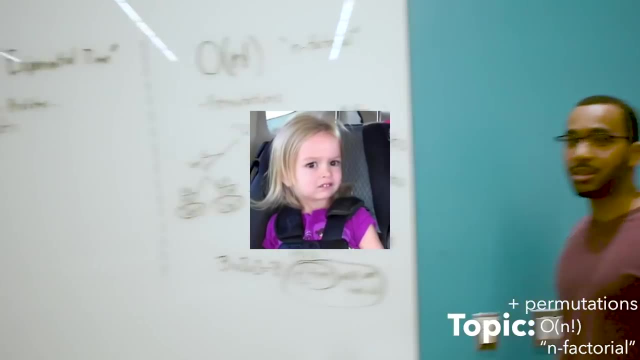 So this is called N factorial and you'll see this time- complexity when calculating things like permutations. So here's a really good example. Do you think you could see it? Can you see it? You can see it, Cool. Okay, so we have cat. 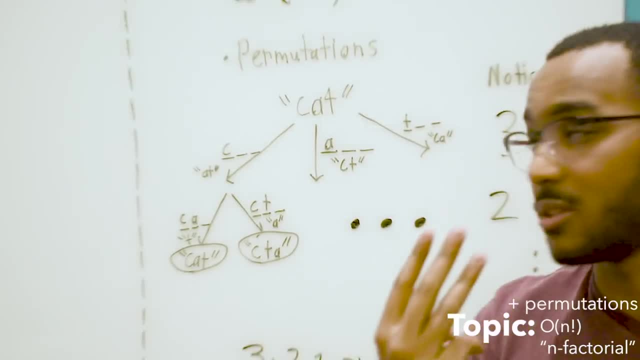 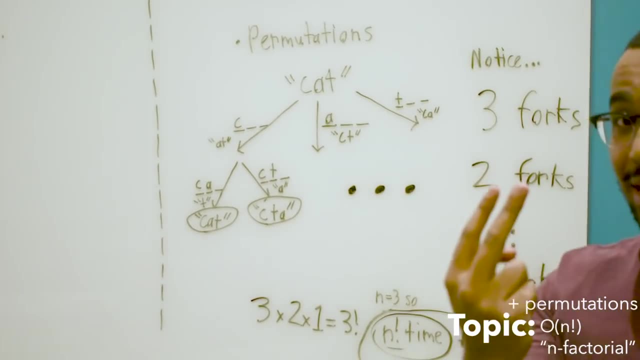 So what we need to do is we have three elements to place. Once we place the first letter of each, we have two leftover elements, and now we need to place two elements three times. So let me not get too much into specifics. What you really need to see here. 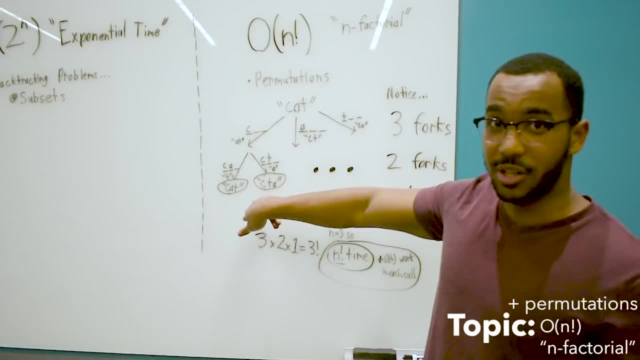 do you see how there's three forks here? Do you see how there's two forks here? So what you need to notice is that for each of these three levels, we're going to be forking twice. For each of these twice forked levels. 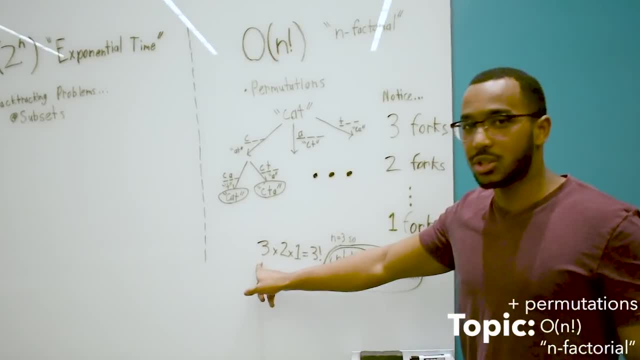 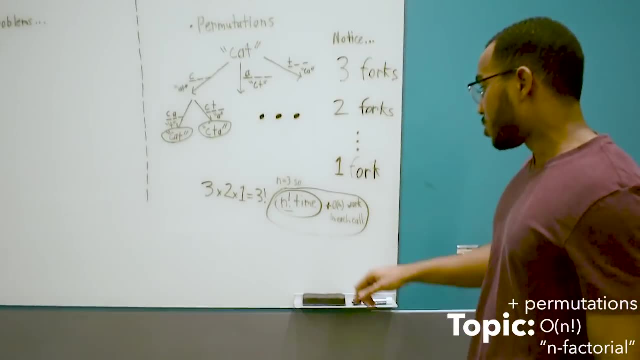 we're going to be forking once. So what does this look like? It looks like three. It looks like three times two times one. What is three times two times one? That's three factorial. So this is why we get the N factorial time here. 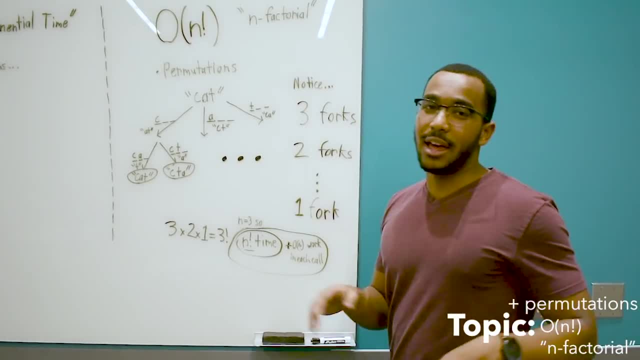 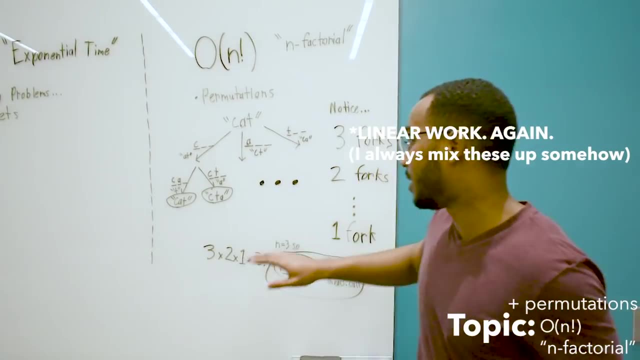 for the permutation problem And the reason. and also it's actually N times N factorial, because if we do constant amount of work to copy the string over in each of these N factorial calls, that's like it depends how much work you're doing in each call. 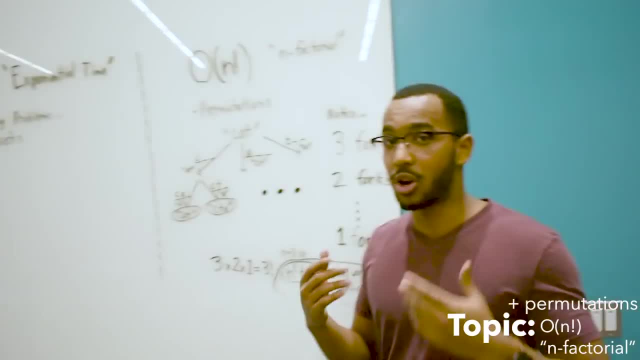 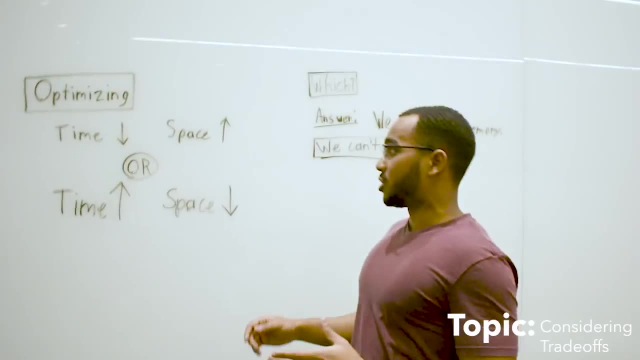 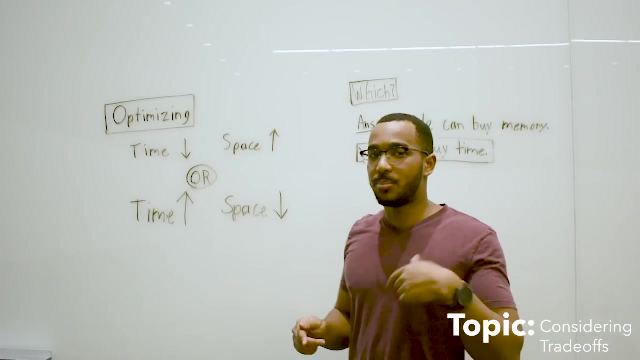 but there's going to be N factorial permutations and N factorial calls, which follows this pattern right here. So whenever we're optimizing solutions like this, normally a pattern you'll see is: you can lower the time complexity and up the space complexity. You can store more space. 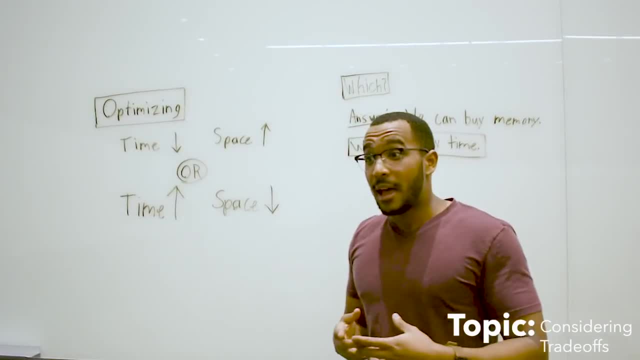 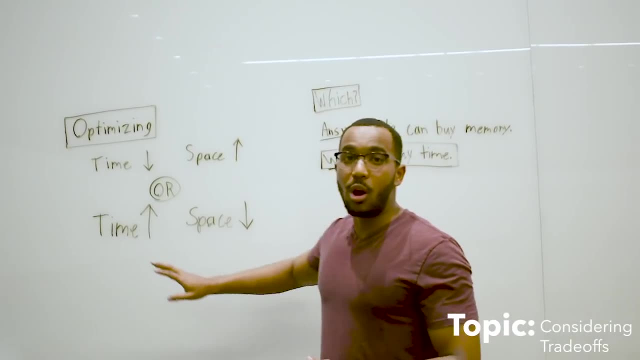 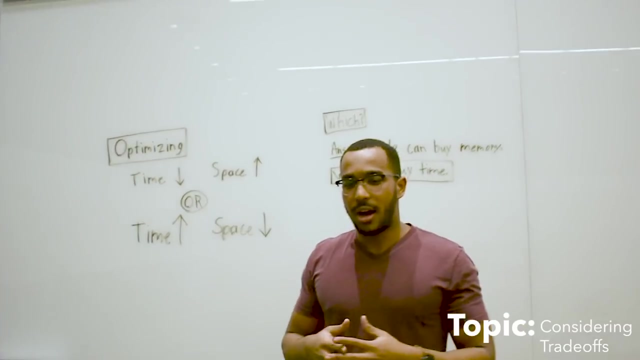 and store more meta information about your problem, And then you can lower how fast your algorithm runs because you know more about the array you're working on or something else, And then you also can increase the time complexity but also lower the space. So you do more work and do things and take longer. 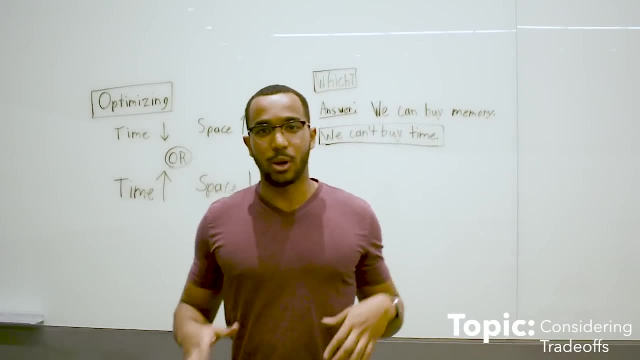 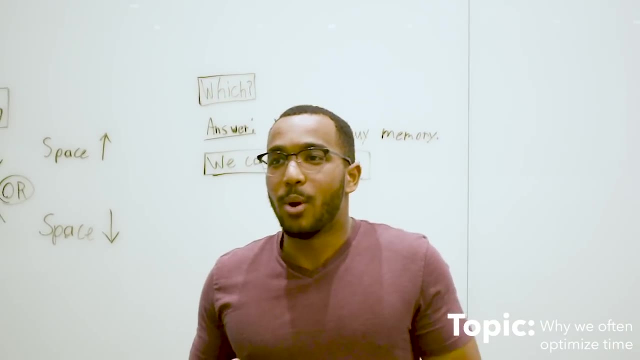 but you keep less auxiliary space. So which one is better, Which one makes more sense? So sort of the answer is: we can buy memory but we can't buy time. So in a production setting, in most settings, it would make more sense. 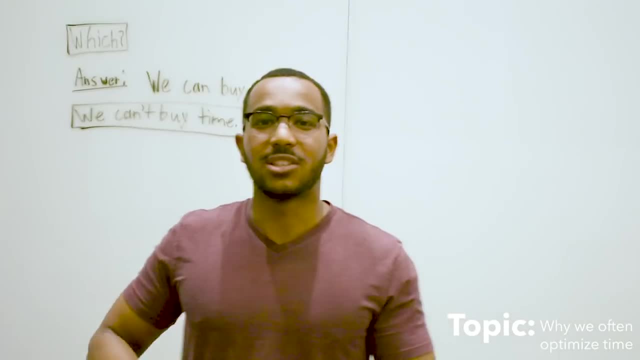 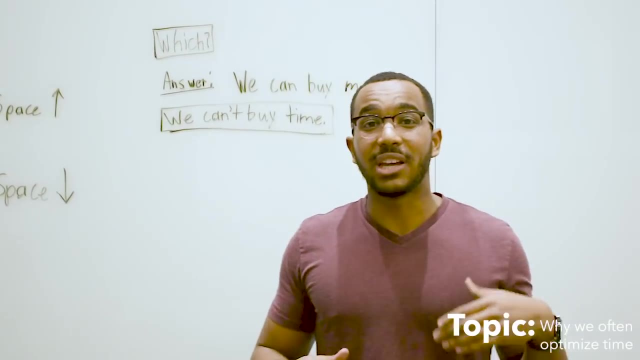 because we always can buy more servers. We can buy more instances of computing power, but you can't buy time. So what you'll find most often is the best trade-off is to increase the space and lower the time, because you want things to run fast. 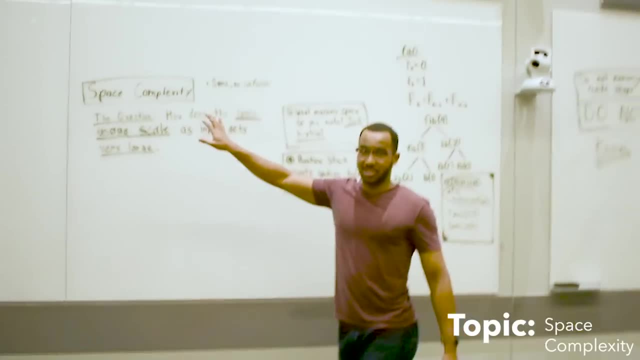 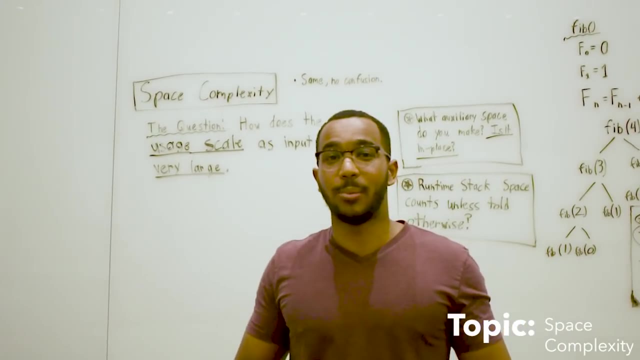 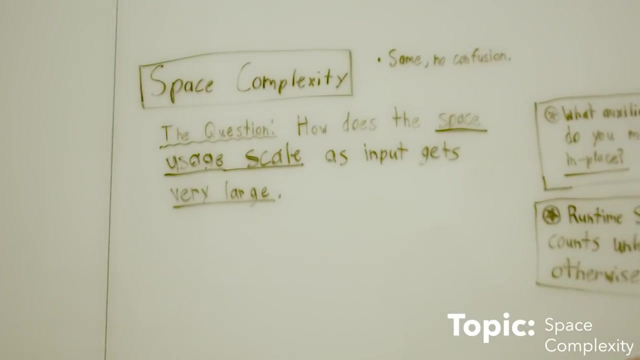 So, moving on, we have space complexity, And this is where some people get confused. Space complexity is exactly the same thing as time complexity. The only thing that changes is the question we're asking. So here, the question we ask is: how does the space usage of our algorithm? 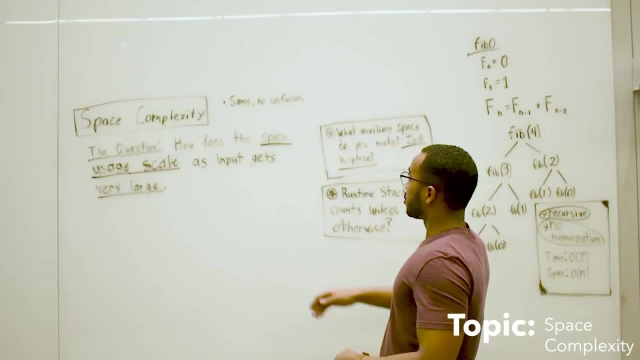 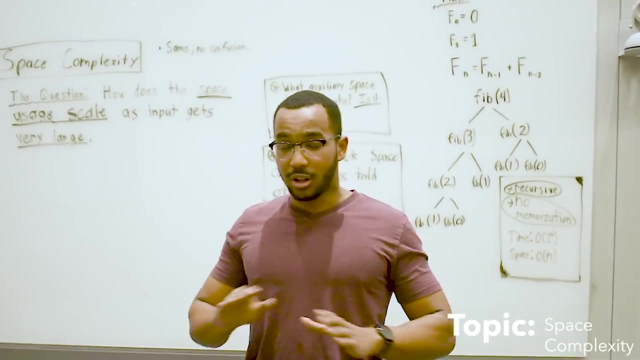 change as input becomes very large. So it's the same thing. There's no confusion. We still have constant time, We still have linear space, We still have log n space. We have all of these same complexities, just our question changes. 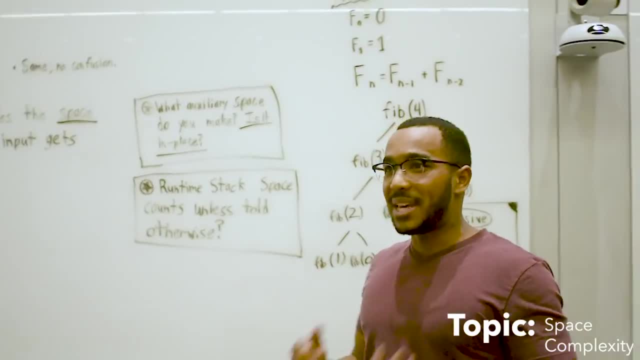 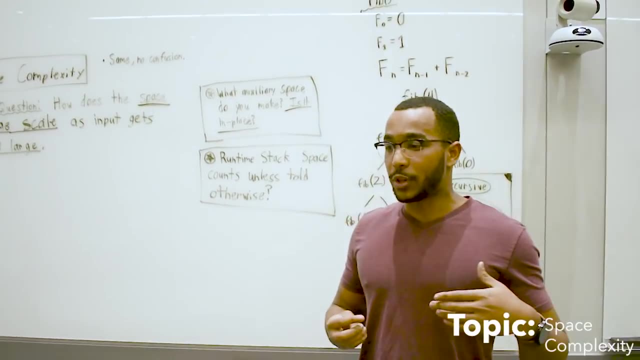 So the biggest question to ask is: what space does your program create? Do you create a single array of n elements? Then you have linear space. Do you create log n elements? Do you create n squared? Do you have an n by n matrix? 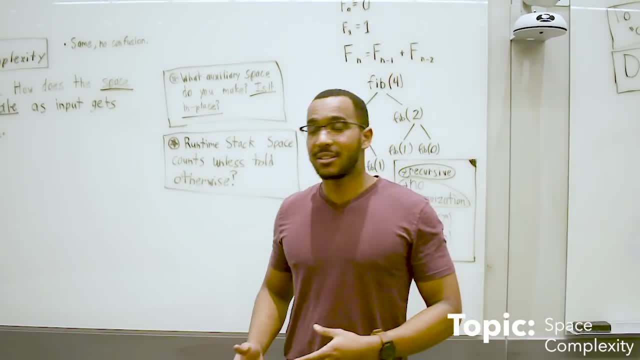 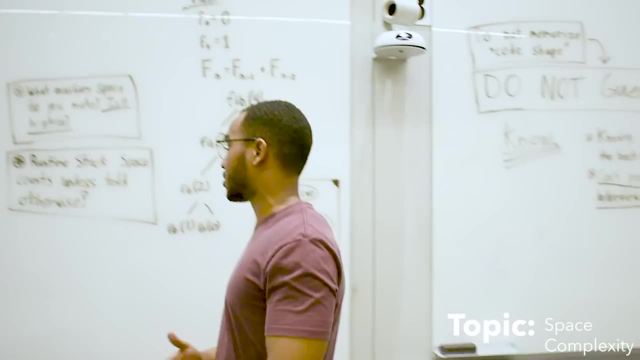 that you're copying over instead of doing something in place. Those are the questions asked. What auxiliary space does your algorithm use, Or is it in place? Does it just use constant space? And then also the runtime stack counts As part of our space complexity. 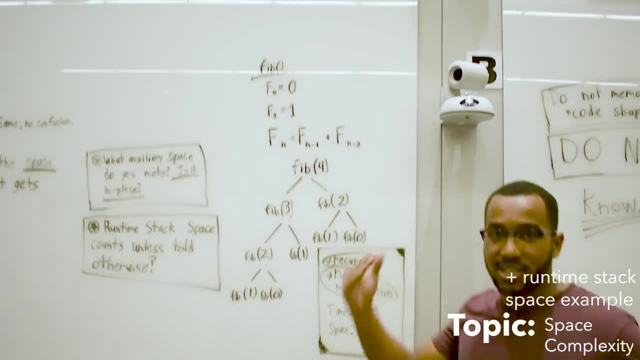 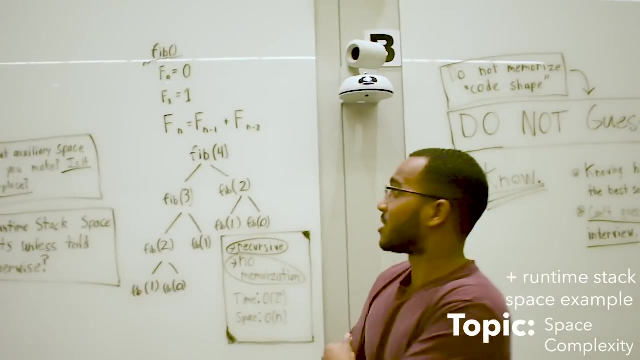 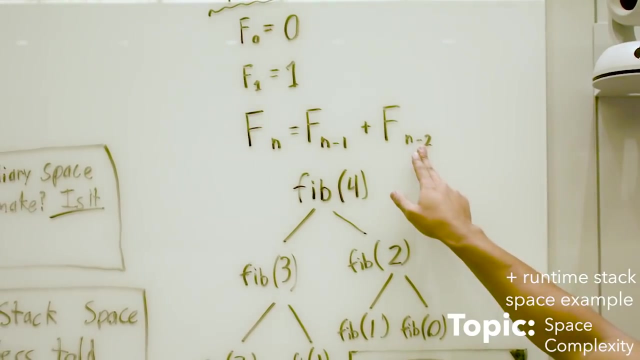 So here's an example of the runtime stack counting. So there's a famous thing called the Fibonacci sequence, And it's defined recursively as the nth element is the one element behind that nth element plus two elements behind that nth element, And then the base cases are: 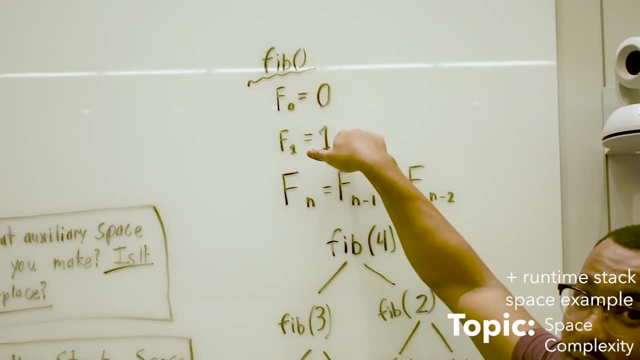 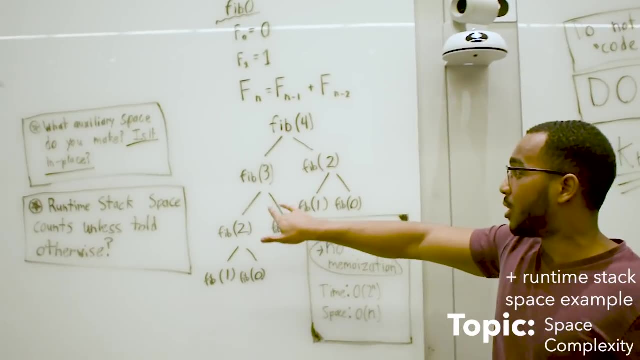 the zeroth element is worth zero, and the first element is one. So this is what the recursion tree looks like. If I want to know fib four, I ask myself fib three, fib two. If I want to know this, I ask myself two, one. 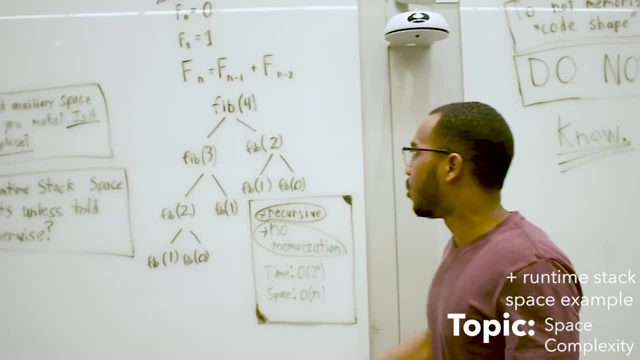 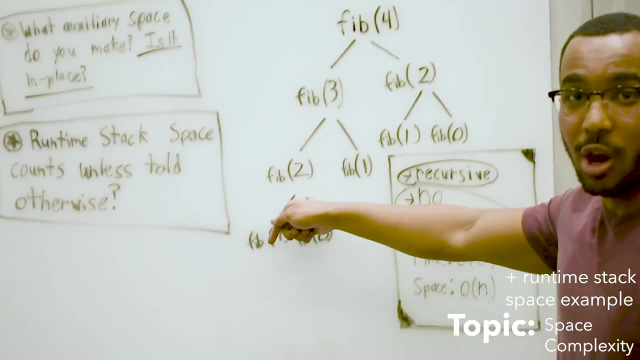 If I want to know two, I ask myself one and zero. So what do we notice? How deep does the call stack go? Because this is sort of like backtracking. We'll go deep And once we solve this problem, the call stack is going to remove these. 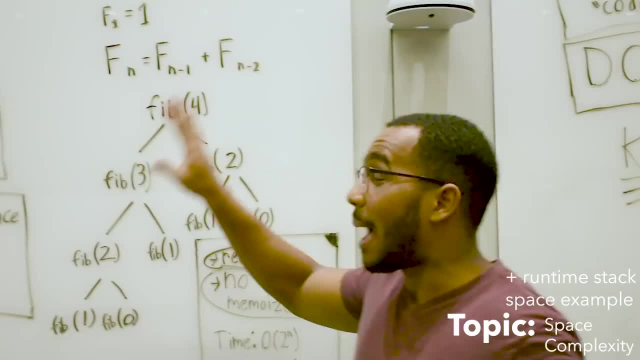 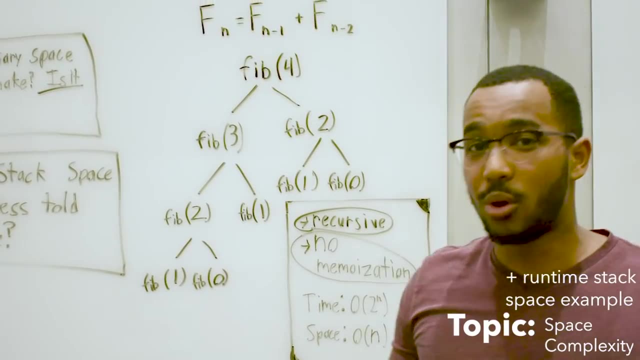 It's going to remove this, It's going to remove that And at max, how many calls do we have on the stack? At max? we can see we have four levels. We're going to have four levels on the stack And four looks familiar. 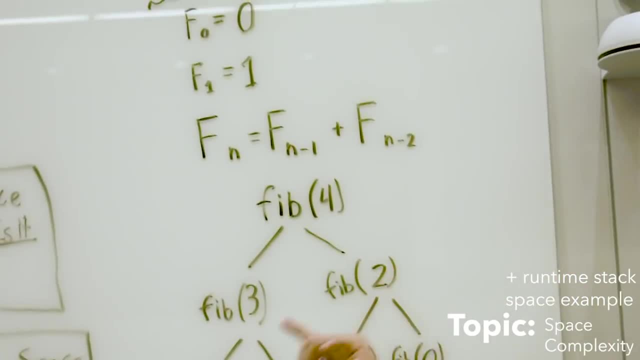 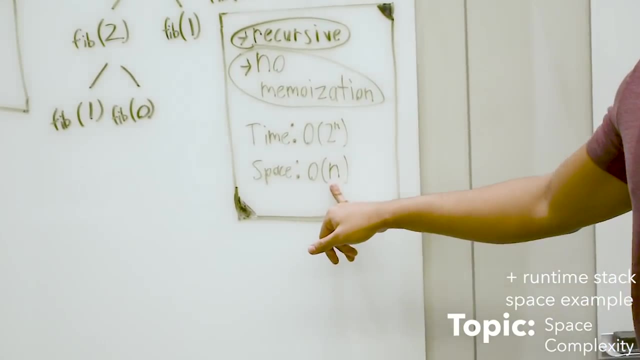 Where do we see four? We see four is the input. Our input n is four. So what does our space complexity become? We see that our space complexity becomes O of n. It becomes linear Because at max we're going to have n calls on the call stack. 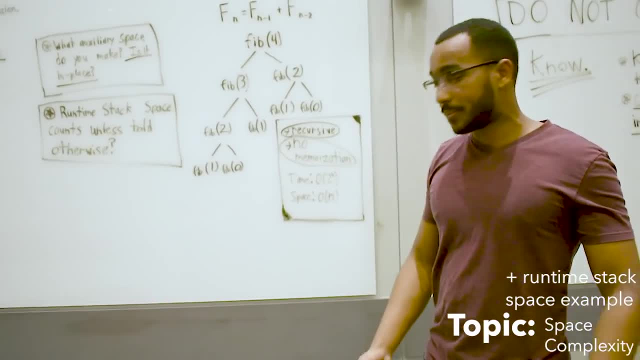 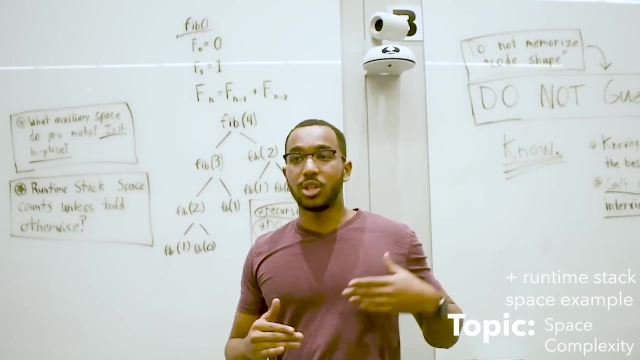 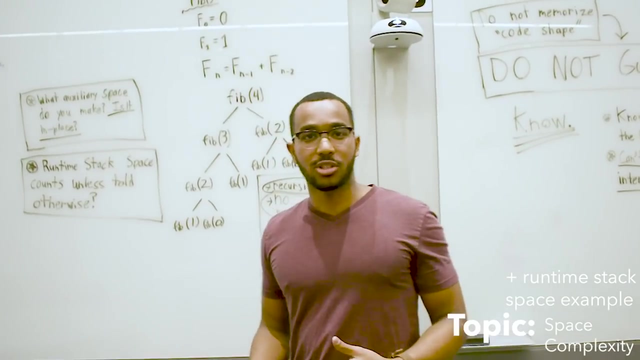 for this recursion. So if sometimes interviewers will not count stack space, that's something you should just explicitly ask. Should I include that in the space complexity, The amount of space that recursion takes up on the call stack? So that's something to keep in mind as well. 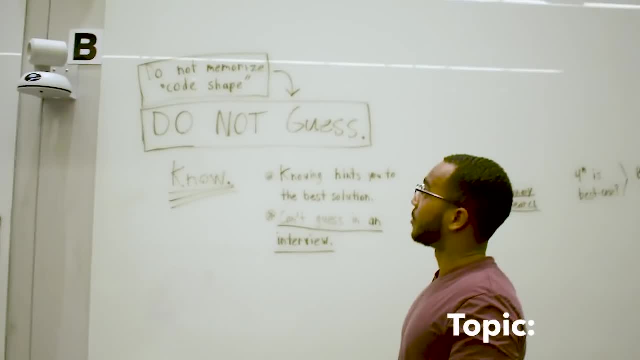 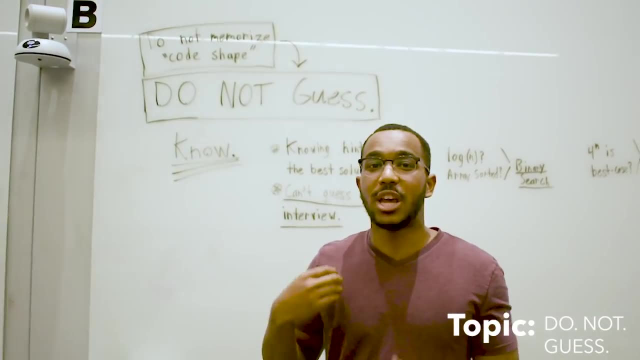 So this is a very huge point. The number one thing is what we'll do. when I first learned big O notation, I would try to memorize the shape of code. I'd see two for loops and I'd say n squared. I'd see one for loop, I'd say n. 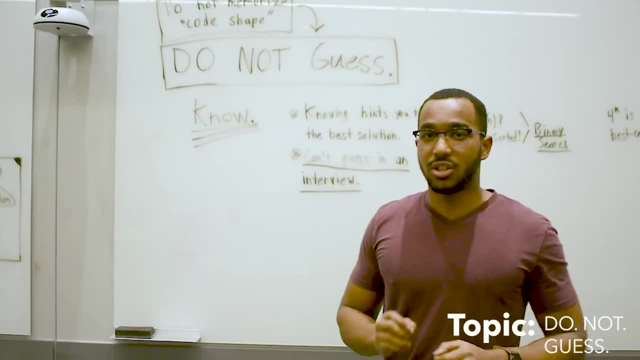 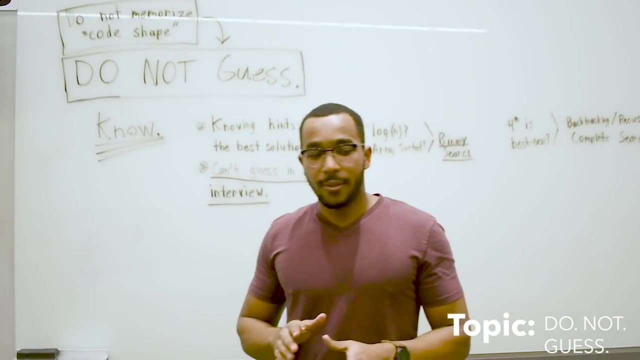 But that's not what you should do. Don't try to memorize the shape of code, Don't try to guess anything. You need to actually know what's going on, Because, first off, if you know what's going on, it's going to hit you to the solution. 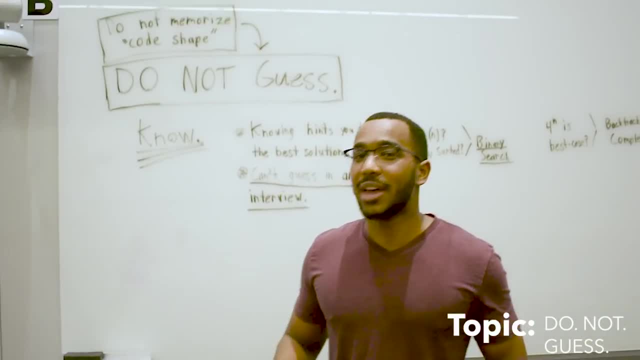 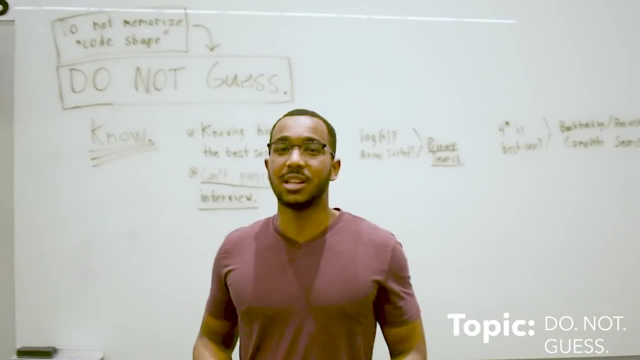 If you know something, best case is log n- then you know that it's going to be something like binary search or something where you're having the search space. So also, secondly, you can't guess. in an interview An interviewer will ask you what is the best case. 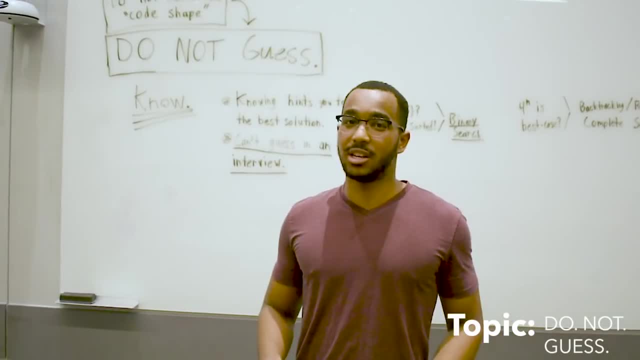 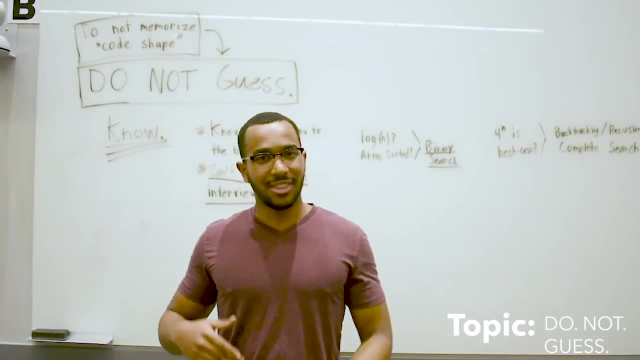 What is the worst case And what is the average case of this? You can't guess in an interview, So don't actually learn the complexities. Try to understand and be flexible. When you're answering a problem, think about it on your own.